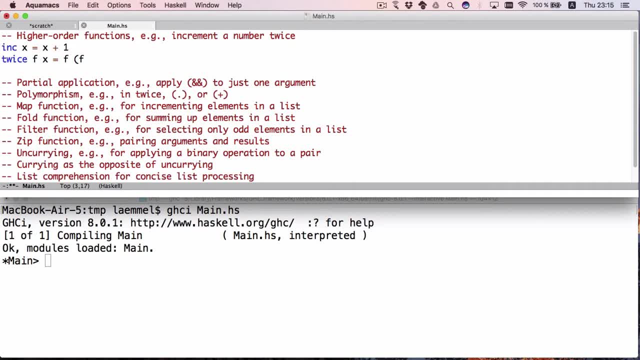 application of second to a second. application of f here to X. Okay, so this should work. We can now apply twice to increment to 40. And it's all fine, Okay. so obviously twice is a higher-order function, because it takes a function as an argument. Okay, and it returns. well, depending on what. 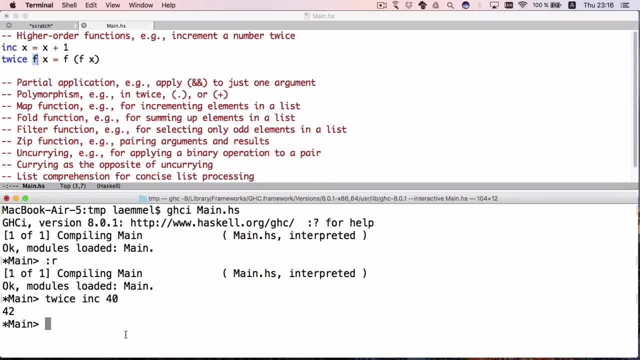 axis, it returns a value. Okay, actually the application of increment is a function, So that means that increment can be applied to a function's value, And again we can have a function f and an argument f as a function value. So this is a function f from a function value that we can also express with the 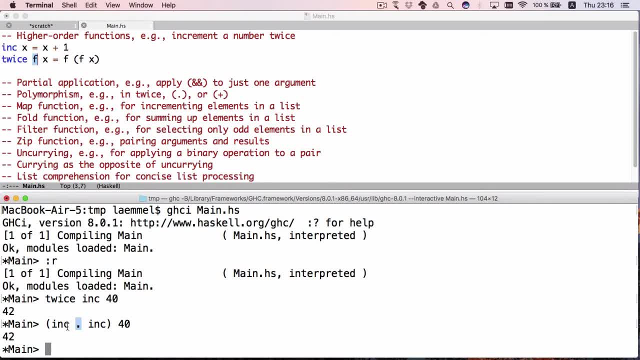 help of function composition. So this pretty much does the same job, right? So here the dot is function composition, and so we compose ink with another ink and again apply it to 40. So which, by the way, we can also use here to rewrite this function composition and apply it to an jeep. 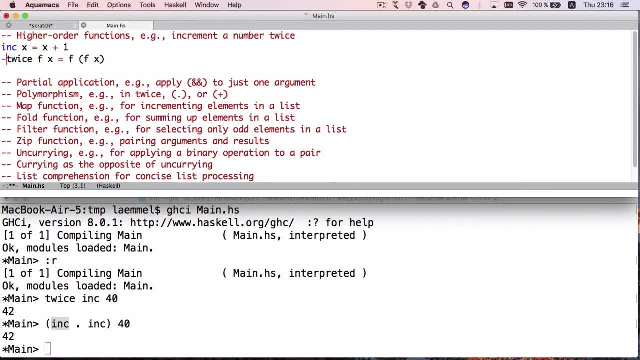 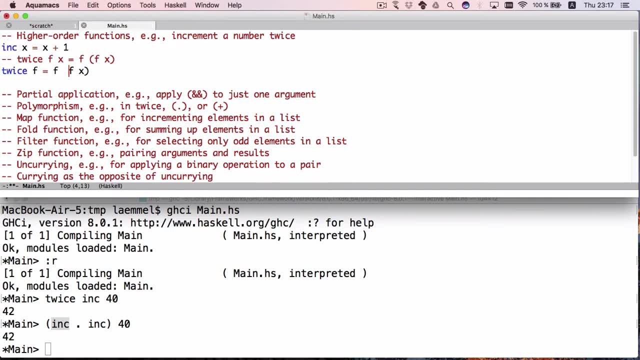 But let's see how we would do it. Of course we can do it in a different way. We can do it in a different way. this definition of twice? okay, so we don't need to take the X explicitly, because we really just need to compose two functions here. well, happens to be. 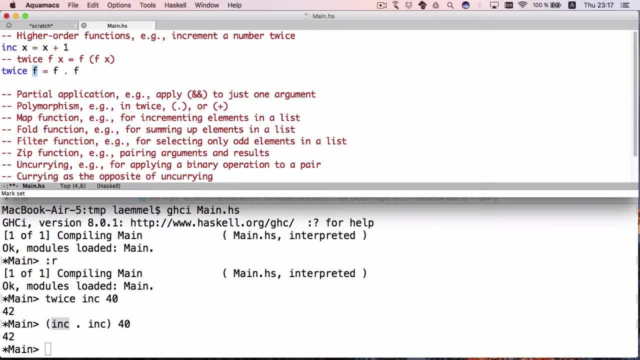 the same function. so not just do we receive a function argument, no, the result of twice is now also function. okay, so we can also do something to make increment look more concise. and this way we come to the second topic, which is closely related to higher-order functions. that is, there is no need here. 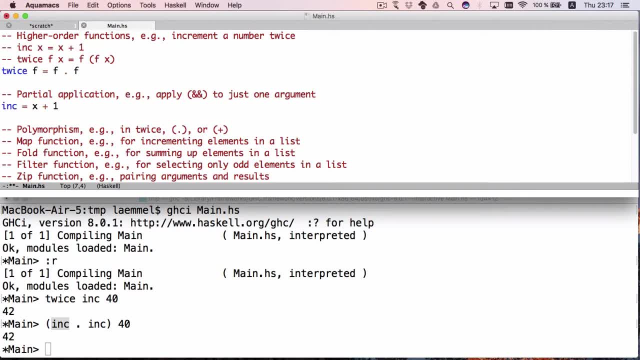 to really take the, the, the, the, we can just form a partial application of addition. so this is basically the prefix form of addition, whereas here we use the infix form of addition and we just say, okay, increment is the same as using addition with the argument with. 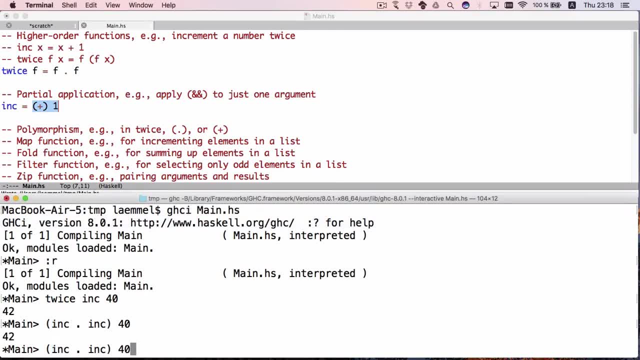 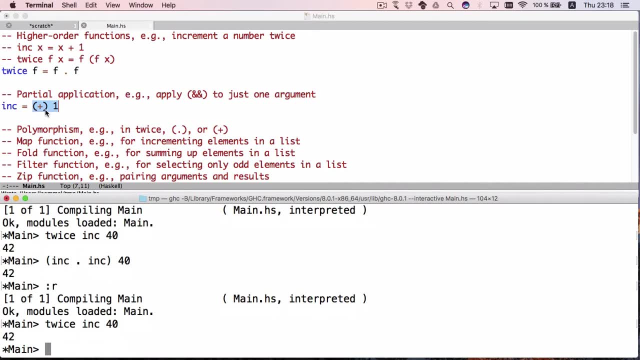 one argument being one. okay, so this also works as before, and in this manner we see how we perform the partial application of addition. right, a full application of addition would be something like 20 plus 21, well, 22, I guess that would be a full application. and now here, what we do is we 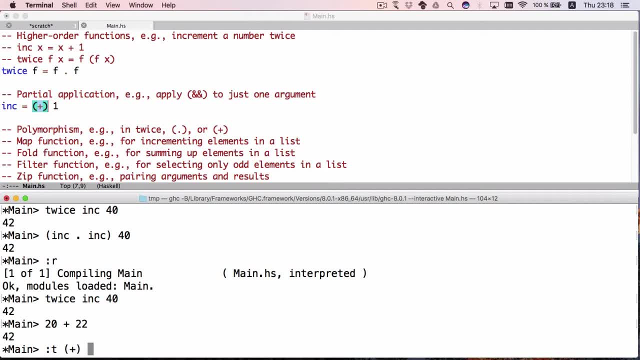 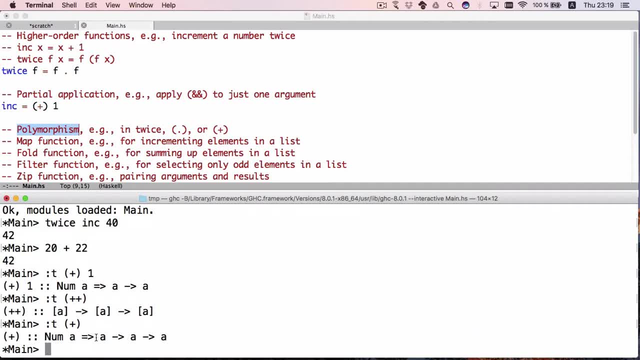 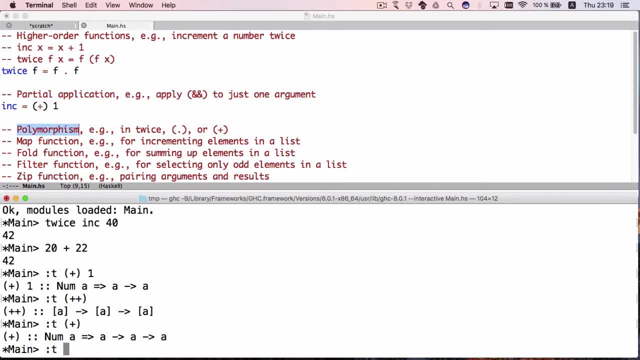 And let's just look at another polymorphic type. Here's the polymorphic type of function composition. Or let's also look at the type of twice. Here's the polymorphic type of twice. By the way, we see that the type is polymorphic when some type here starts in lowercase. 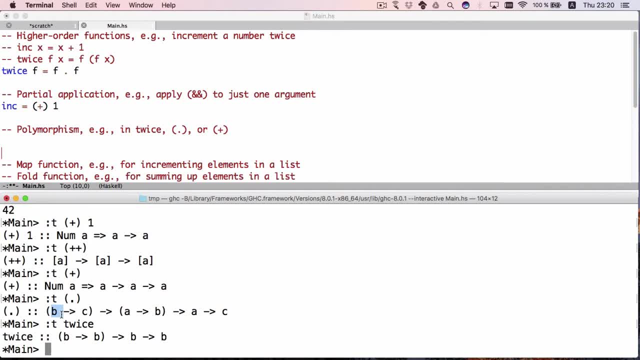 because then we look at the type variable, And this is what makes types polymorphic, All right. so the type of function composition is actually very interesting because it immediately reveals in what order, so to say, the arguments of dot are applied, Since the resulting function of function composition maps an a to a, c. 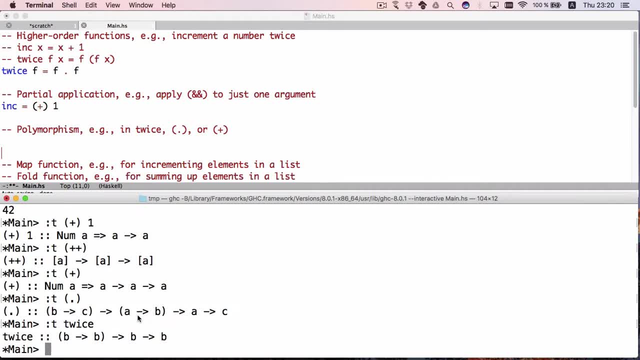 we can see here that obviously the second argument of function composition is a function composition. It's the function that is applied first, because it maps an a to some b, And then the first argument maps that b to the final c. Okay, so this also explains polymorphism. 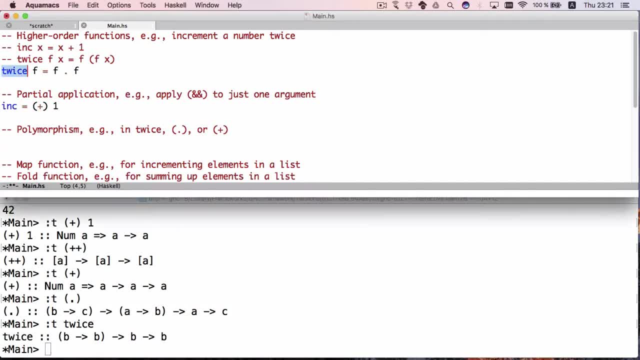 So, by the way, we can of course also explicitly write the type here, And these types are all equivalent Modular renaming, so we can also write a to a and a to a here. It doesn't need to be b. 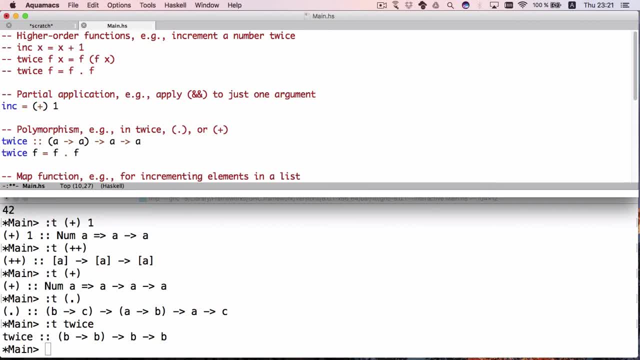 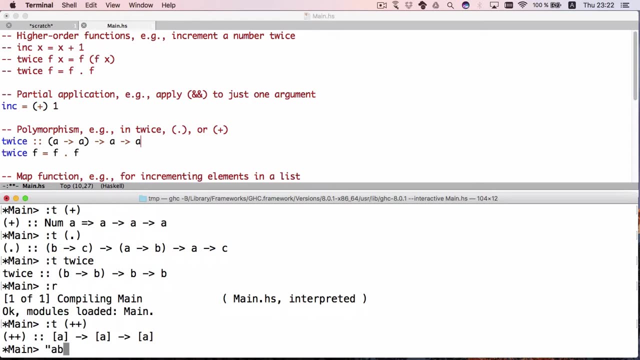 As long as we consistently rename all type variables, it's the same type. Okay, Right, we were also showing the type of concatenation, And This can be used like this, Or it can also be used like this, So that it means it can be used on strings which are lists of characters. 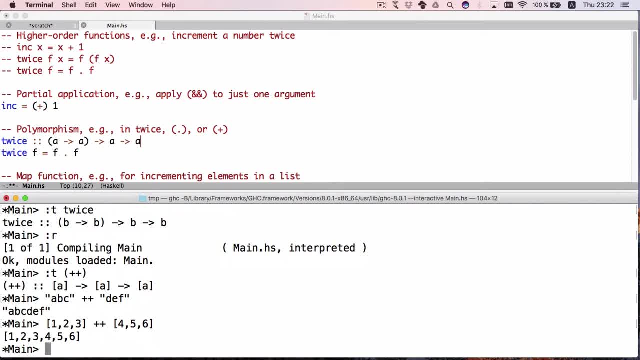 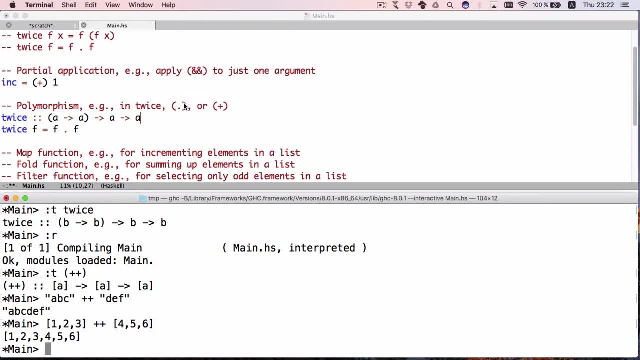 and it can be used on a list of numbers. Okay, so this is just another nice example of a polymorphic function. Okay, so now we've got some basic idea about what it means to be a higher function And what it means to be a polymorphic function. 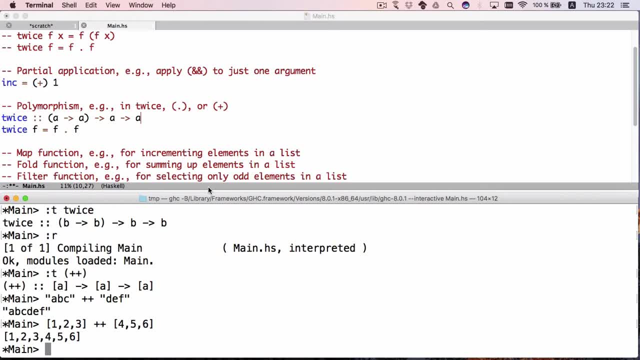 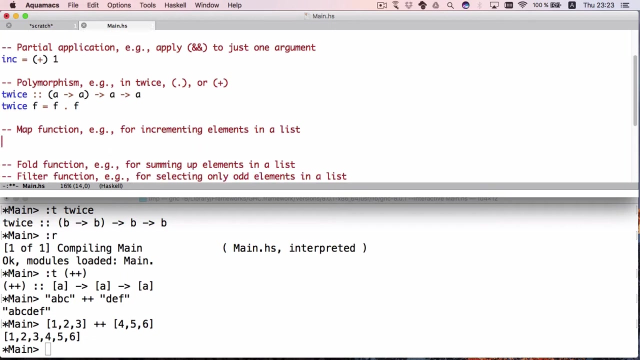 So higher order and polymorphic functions. they show up in particular very naturally in the context of list possessing. So let's start with a function that is not higher order And that is not Polymorphic, And then let's factor it so that we understand the deeper structure. 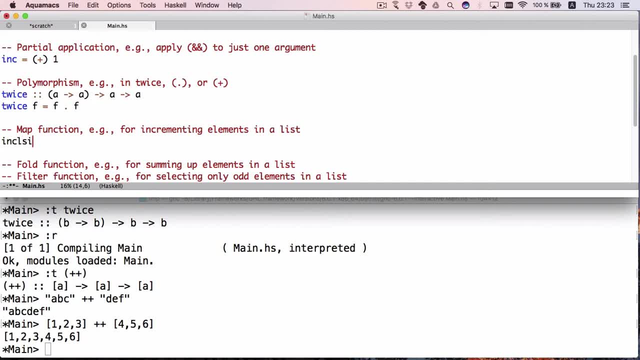 So, for example, we could have a function- incList- which takes a list of ints and returns a list of ints And, as the name suggests, we want to increment all elements in the list. So if you have an x here, an x is there. 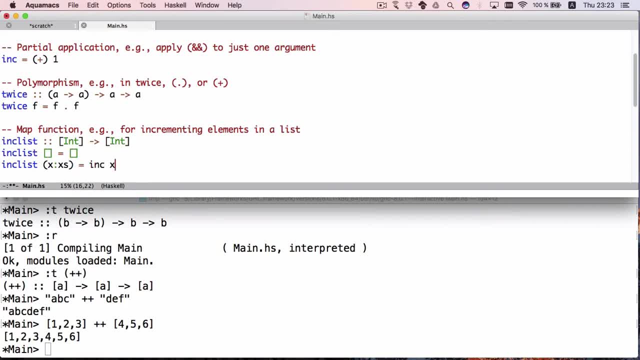 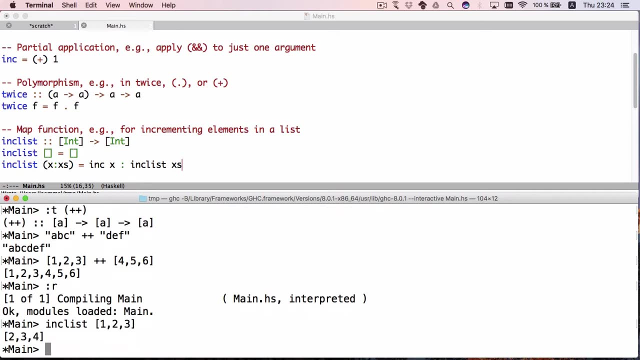 then what we do is we increment x and we recursively increment the list x's. Okay, so far, so good. so we can apply increment list to 1,, 2,, 3, and we should see 2,, 3, 4.. Now 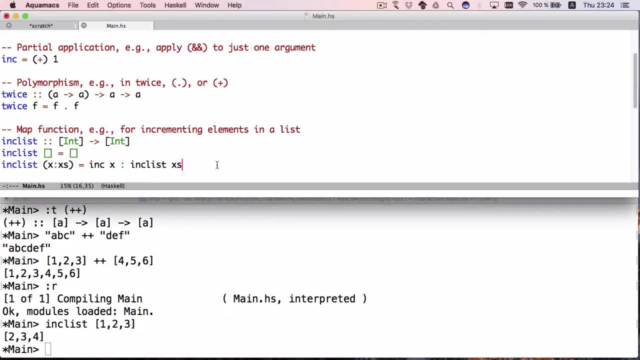 of course this function is. it contains, if you like, border plate code, in the sense that we're doing things that we are likely to do all the time in very similar situation. so what we do here is we say, okay, if we got the empty list, we return the empty list, and then what? 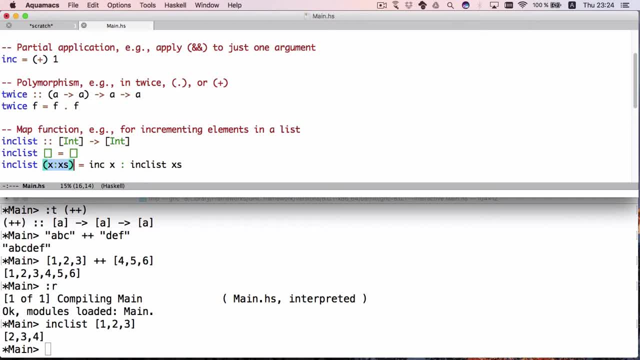 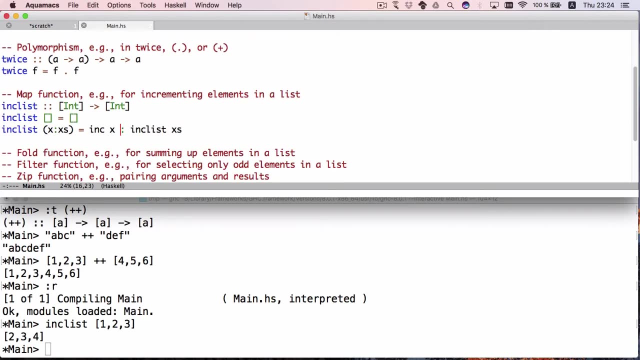 we say here: if we got the non-empty list, well then we do something with the head of the list and then we recursively process with the same function- the tail of the list- and then we just put together these two results. as you can imagine, there are tons of functions. 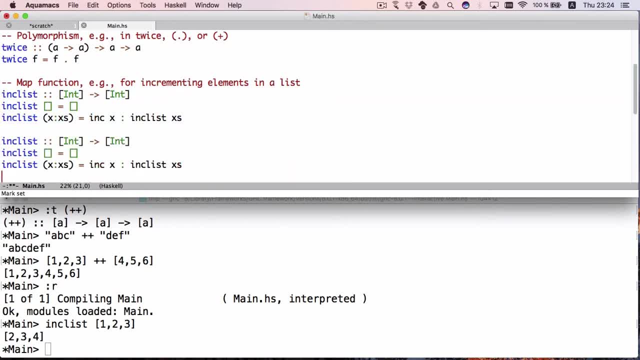 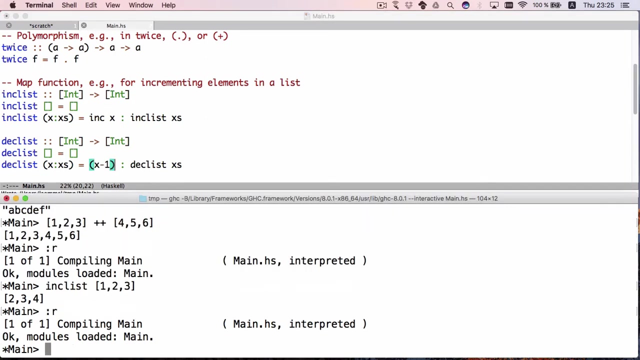 that are like this. I mean, just imagine you want to instead decrement all elements of the list. then you start to write essentially the same function and just that. you here in this place, you will write something else. okay, also works. decklist 1,, 2, 3. 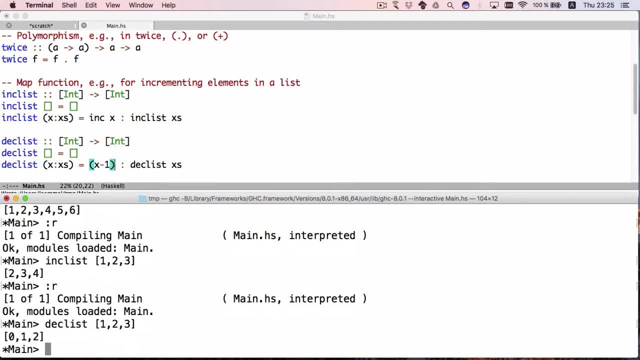 we've got as a result. now, the map function is a high-order function that allows us to capture the commonality of these situations. so let me show this so we can use map and apply it to ink and then apply it to this list, and we get exactly the same result as with the. 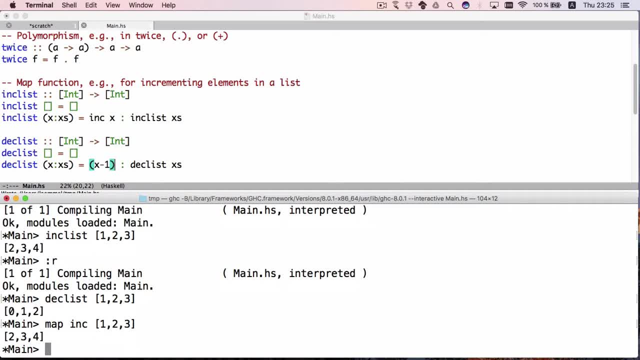 in list function, except that we didn't need to even define any function. we could just right away reuse our per element increment function and that's it. and so, of course, the question is: how does this map look like? how does this map look like? how can we define it? 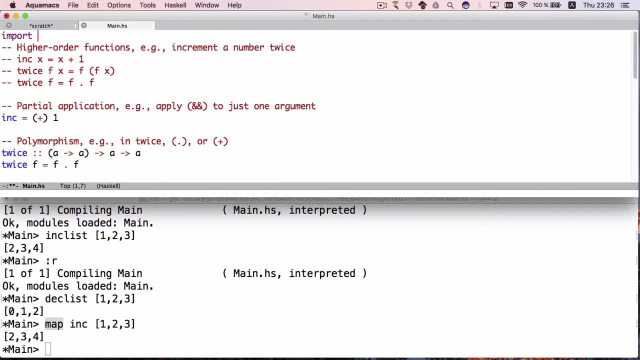 well, in order to define it, we should actually remove it from the import list. so because it's, of course, in Haskell's prelude. so if you want to go and define it ourselves, we better hide it. so map, as we see in this example, takes a function. 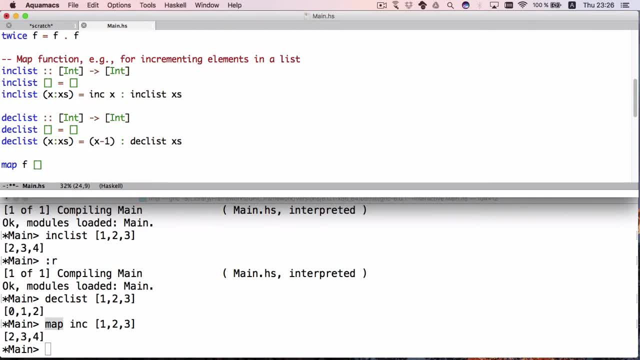 and takes a list and of course, if we apply it to the empty list and of course if we apply it to the empty list, we get the empty list. if we apply map to the non-empty list, then what we do is we apply the argument function f to x. 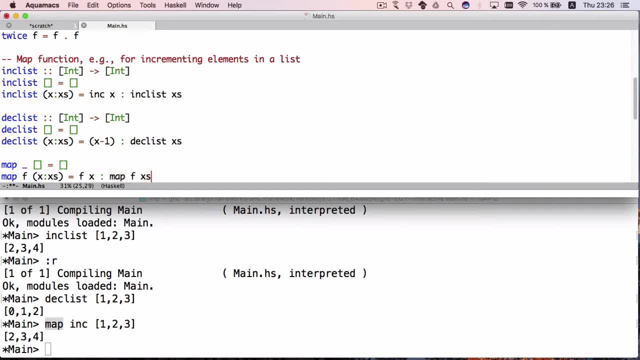 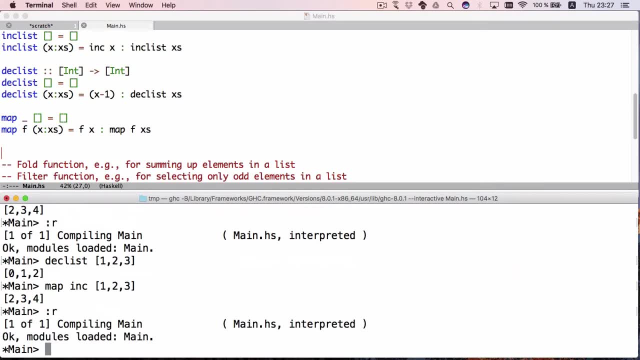 and we apply map f to the rest of the list. okay, so let's just see that it still works. yes, and we can also look at the type of map. yes, and we can also look at the type of map. this is the type of map, so let's copy it here. 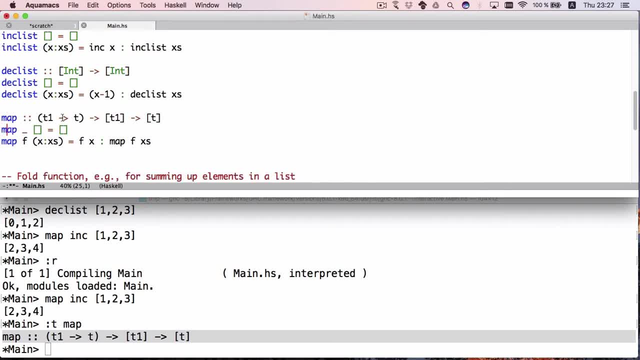 well, and actually let's make it nicer. so we replace t1 by a and t by b. makes it a little bit more readable. so now it's clear what happens. given a function from a to b and given a list of a's, we return a list of b's. 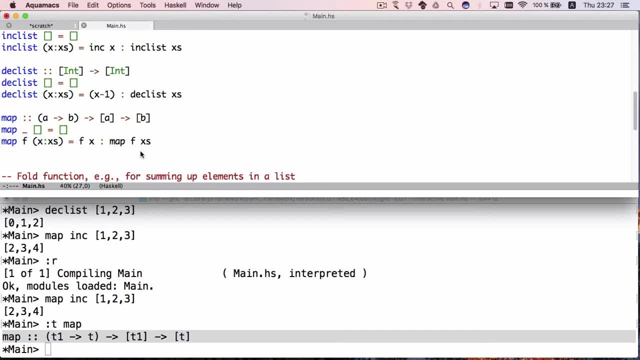 well with increment. we didn't do that. we didn't even exploit the fact that argument and result can be of different types. but let's look at a different example. so let's, for example, say we want to apply odd, which is the predicate for determining whether a number is odd. 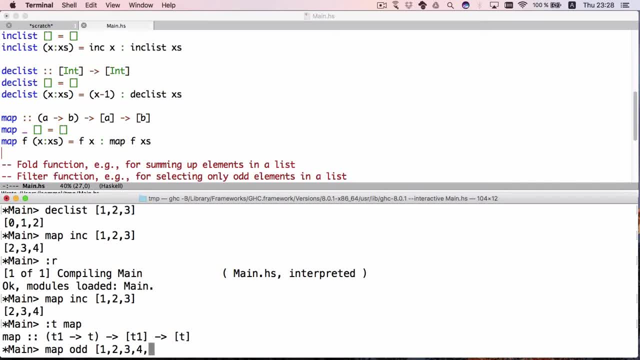 and we applied 1,, 2,, 3,, 4, 5. yes, that also works. so we basically have mapped odd over the list 1,, 2,, 3,, 4, 5, thereby computing Boolean values that describe whether the original elements. 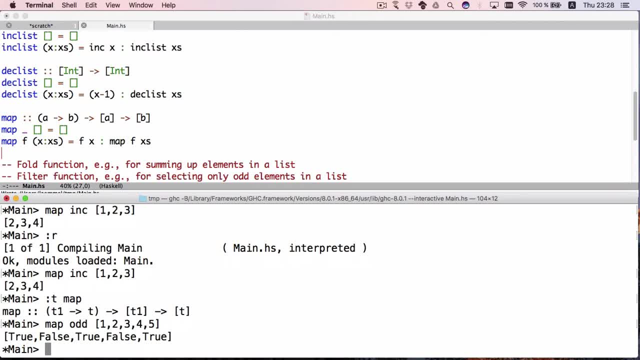 were odd or not right. so this is the map function and it's quite obviously a higher order function because it takes a function to apply to each element and then it takes a list and returns a list. it's quite obviously also a polymorphic function because we don't want to be constrained. 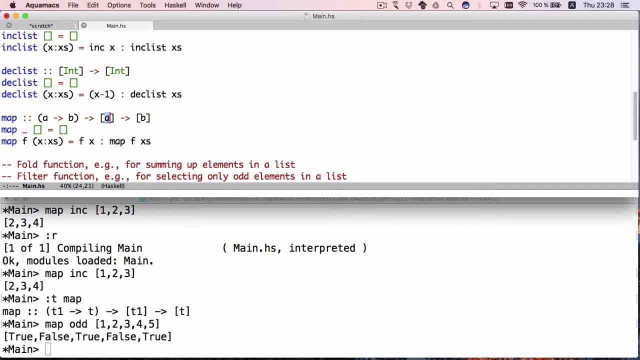 in the element type of the input list and also not in the result type of the per element function here. and, by the way, just to make clear that we can define INCLIST in terms of map, we could also have written INCLIST prime here, and that's basically the new definition. 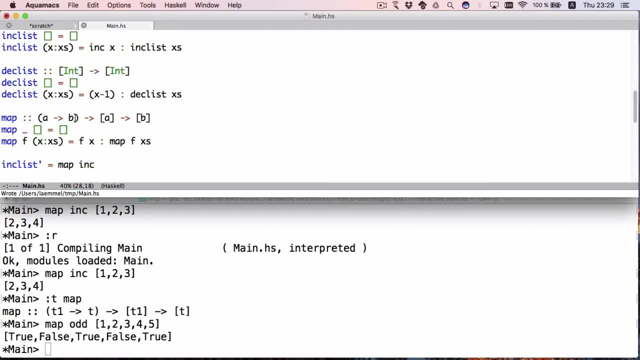 so we can also give it a name. but maybe we don't even need it, this new name, if we know it's just the application of map. ok, so of course DECLIST prime would be something like MAP DEC if we had DEC DEFINE. so ok, let's just define DEC here also. 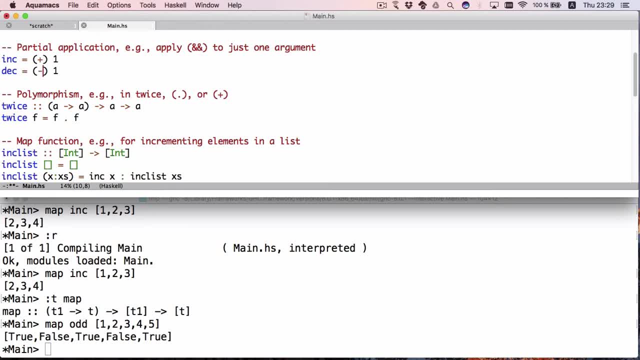 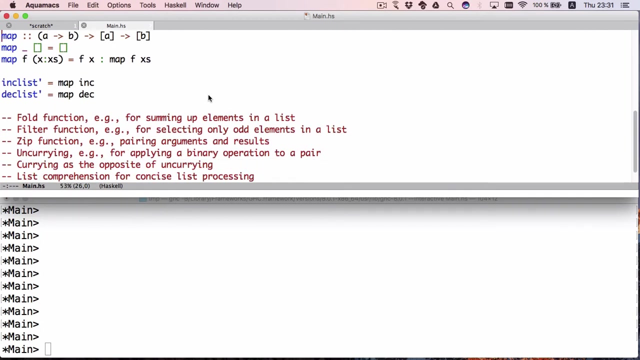 and, by the way, this: we cannot do like this, because obviously this would be the first argument of subtraction. so we would not decrement, but rather we would subtract the remaining argument from the from one. so what we could do is we could do this and that. now let's look at a similar 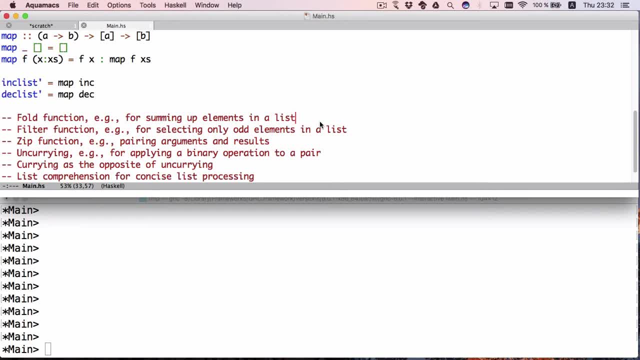 problem. we don't want to map a function over a given list to get another list. rather, we want to sort of what's called fold over list so that we get one result. let's again start with a non higher order, non polymorphic formulation. so, for example, let's say: 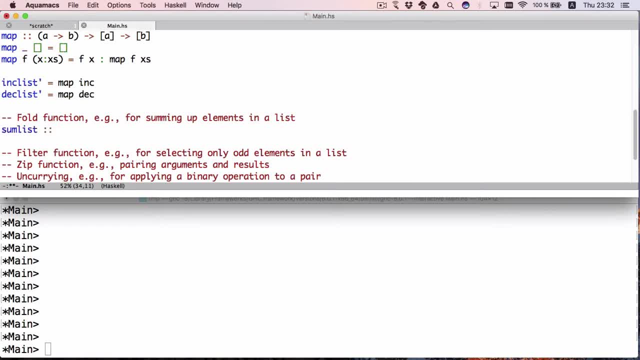 we want to sum up a list, so let's do this. and we do this, of course, by saying that the sum of an empty list is 0 and the sum of a non empty list is x plus the sum list of the remaining elements. and, by the way, 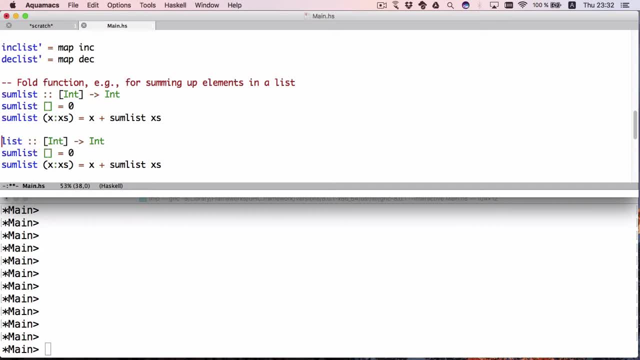 just to show you another function that looks very similar. let's also take prod list, so that we compute the product of all elements in the list, and here we assume that the product of the empty list is 1 and we apply multiplication here. okay, so for example: 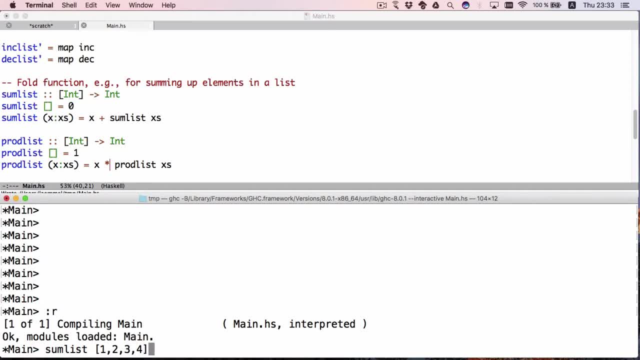 sum list of 1, 2, 3, 4 is 10 and prod list of 1, 2, 3, 4 is 24, or 1, 2, 3, 4, 5 is 120, because it's the factorial of 5. 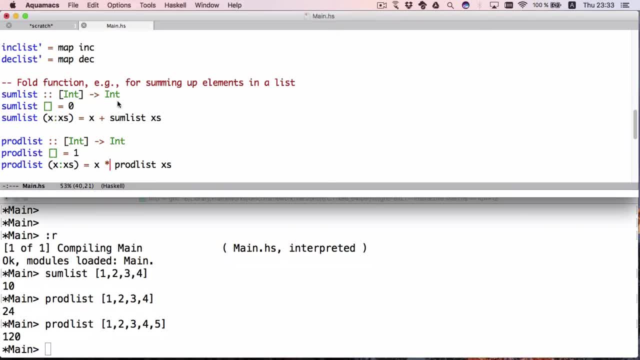 now again, these functions are very similar in their structure and it's sort of unsatisfactory to write such code that seems to follow a pattern. so in function programming we really try to extract patterns into higher order functions, and this is very easy in this case. so 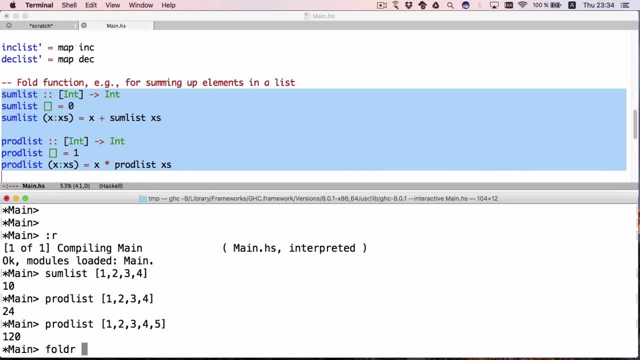 what we do is we can just do a fold. in fact, there are different kinds of folds. we use what's called a right dissociative fold. right dissociative in the sense of the list structure and how we apply a binary operation. so we say, okay, we apply. 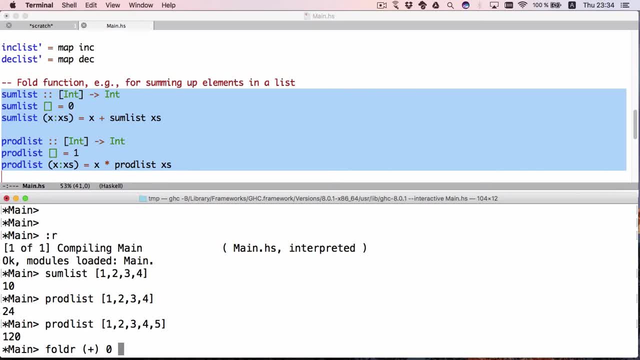 addition, and we start from 0, and when we apply this to 1, 2, 3, 4, we get 10, as we were planning. if we instead apply multiplication and 1 here, we get 24, as in the case of prod list. so this means we have obviously 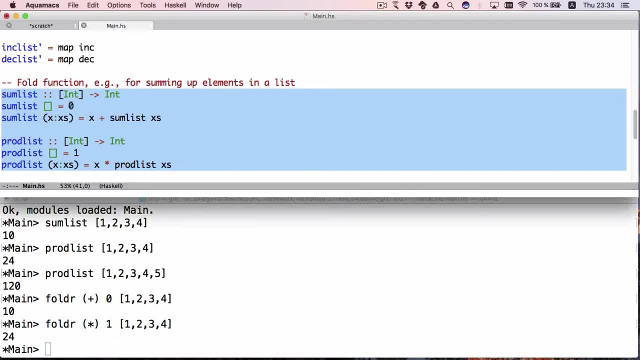 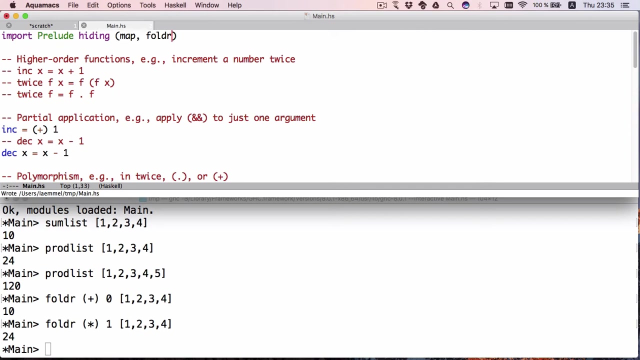 factored the pattern of applying a binary operation on the elements of a list, including the specification of an element to start from. so of course, we again want to know how fold or actually is programmed and we remove it from the prelude. okay, and let's go here and let's try. 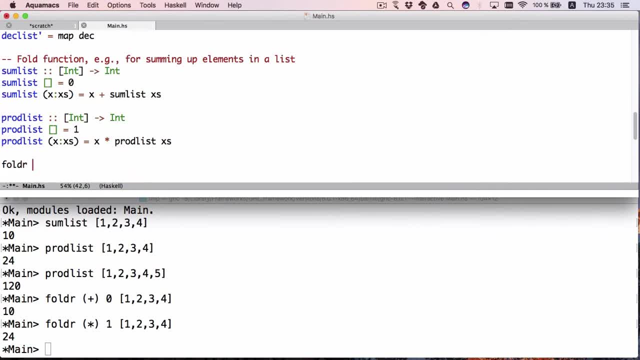 to find it so. fold or take some function f and take some initial element, and when we apply it to the empty list, well, we pretty much don't have any other choice than returning z. when we have a non empty list, then what we need to do is: 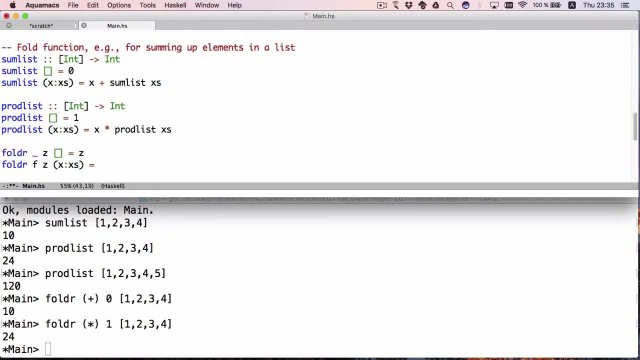 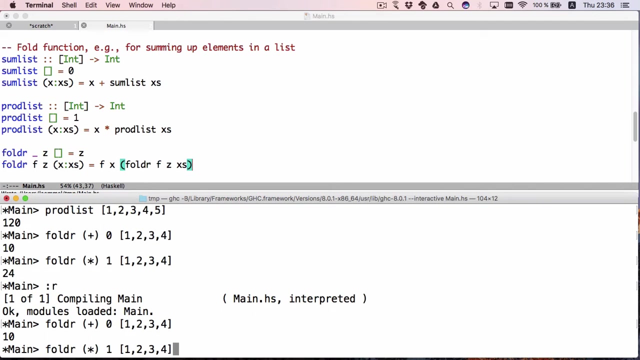 of course we need to somehow recurse and we also somehow need to process x. so what we do here is we apply f to x and we carry out the recursive application f- z axis, okay, and so we can still perform addition like this, multiplication like this, and again we might wonder what the type is. 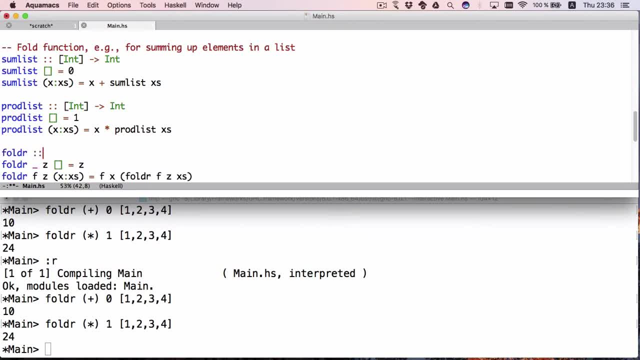 and this time we just try to figure it out ourselves. we could of course also use type inference, so we start from the back. so I mean, obviously we somehow take a list of, let's say, a's so, and we somehow compute an a, and here we take a binary. 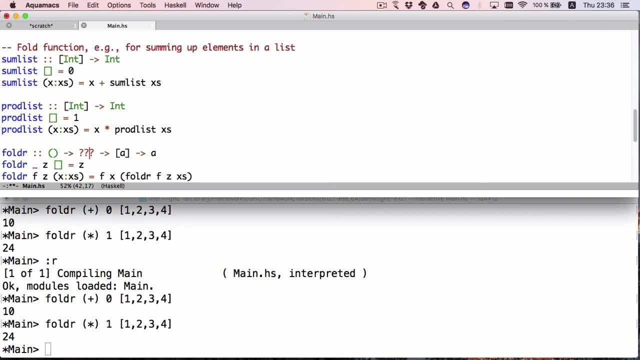 operation on a's okay, and here we also have z a. in fact there is nothing in this definition which forces us that this needs to be the same type as the element type of the incoming list. so we put a b here and then we can put a b here and put a b. 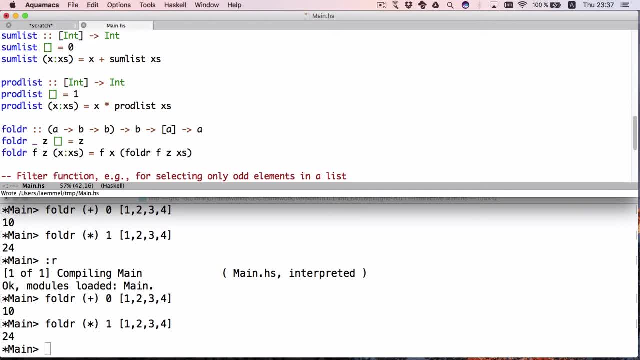 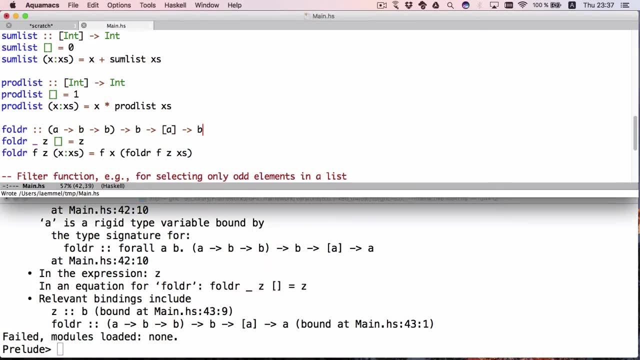 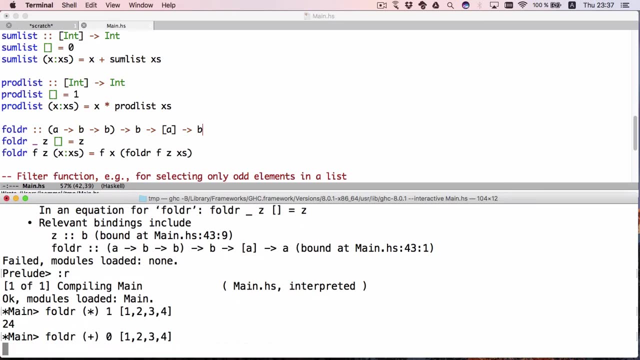 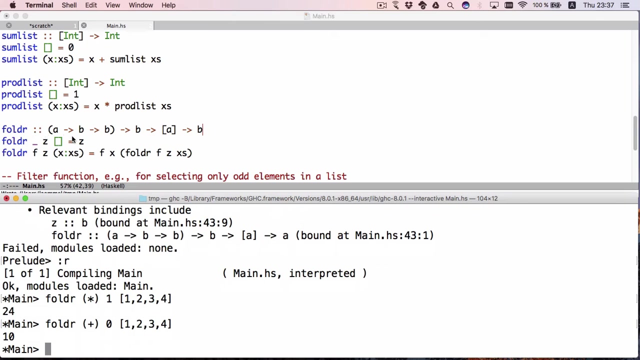 there. this is the most polymorphic type that we can come up for fault. well, we of course also have to put then a, b here. okay, so this still works. yeah, so the key thing is really that the binary operation called r models the repeated application of some binary operation. 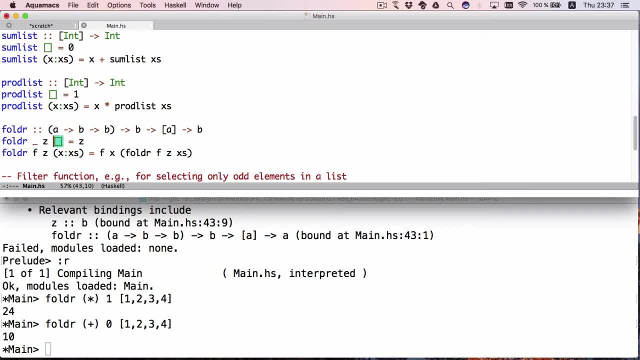 f to the elements of a list, right, so we can also write this differently. we can also, in order to see clearly that f is a binary operation, we can also put it like here in between, and then we see it more clearly. this is how we turn an arbitrary name. 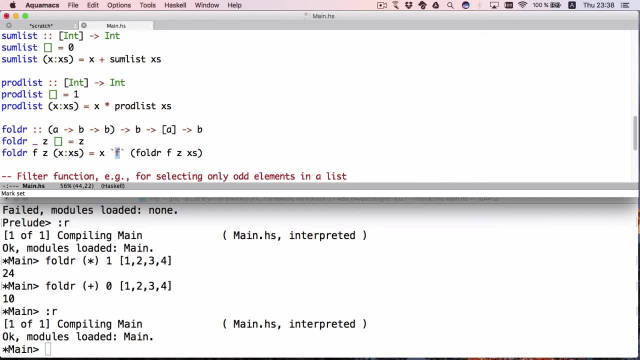 into an infix operator. okay, and again, we can now define some list simply as an application of fault r to addition and zero and prod list is then simply similar application, only that we use multiplication here and one as the initial element. okay, so now we have seen map and. 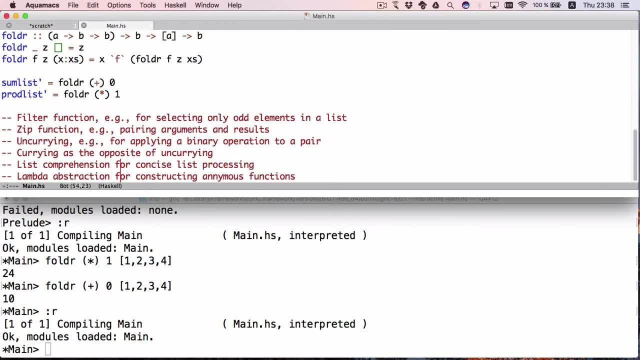 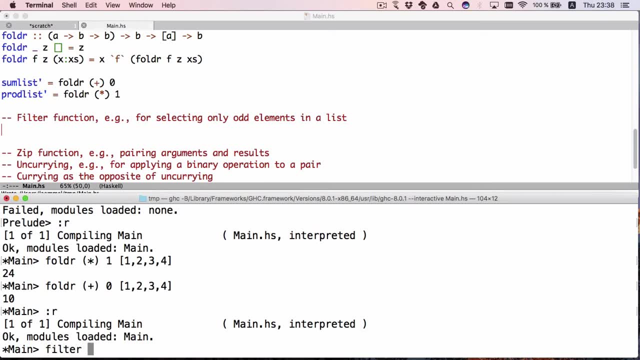 fold and there is one more list possessing high order function in this neighborhood. it's a filter function, so we can just demonstrate it: filter odd on the list one, two, three, four, five. so what it does is it simply determines all elements in a given list that satisfy a given. 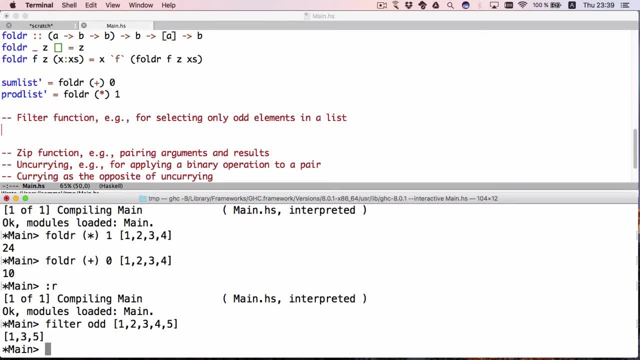 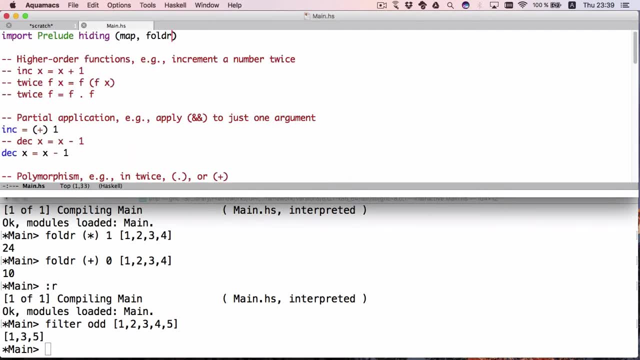 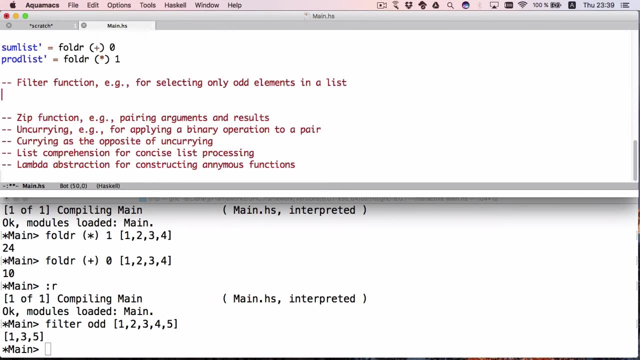 predicate. so we just figure out all the odd elements in the list here. so again you might wonder how we program filter and so well as before we need to remove it here from the prelude, and then we go down here again and we just start thinking, okay. 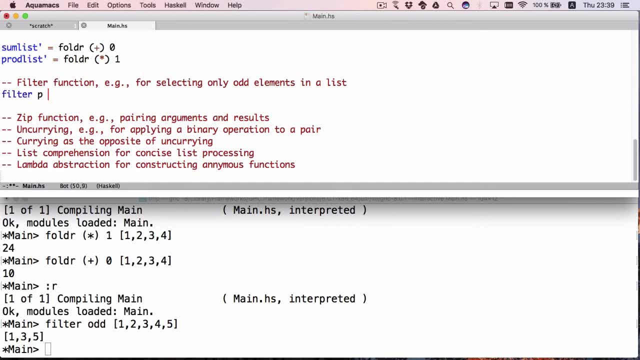 filter takes a predicate, and well, if we apply it to the empty list, then we have no other choice than returning the empty list filter applied to the non empty list. now what we need to do is we need to check whether p applied to x is true. so 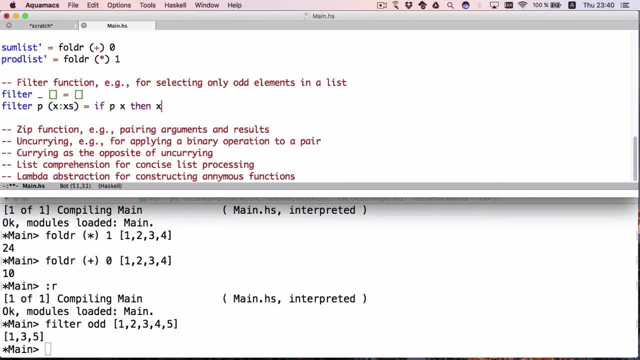 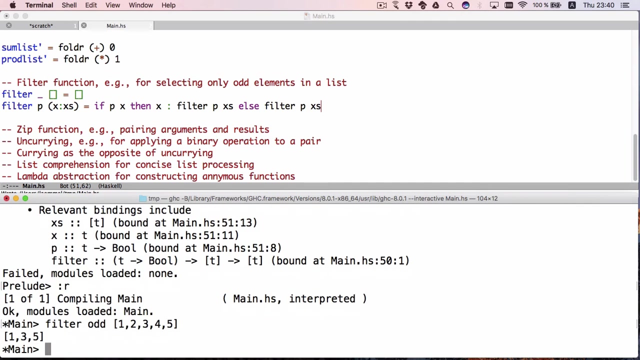 if this is true, well then obviously x needs to go into the result list and we need to filter over the rest of the list. if p applied to x is not true, well then we only need to recurse. okay, okay, so we can still filter. now let's first figure out. 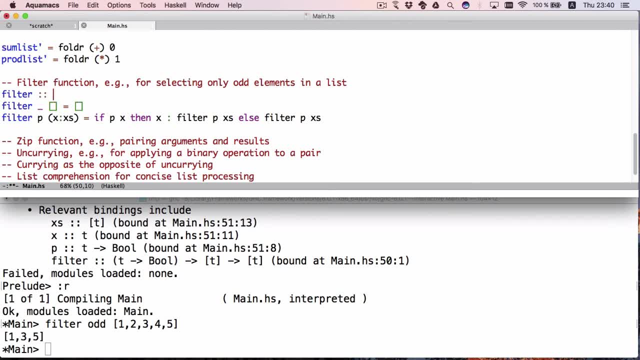 the type. well, the type is, of course, that given a predicate from some type, a to bool does the function, and given some list of a's, we also return a list of a's. now we should do something about the fact that filter p axis shows up twice here. 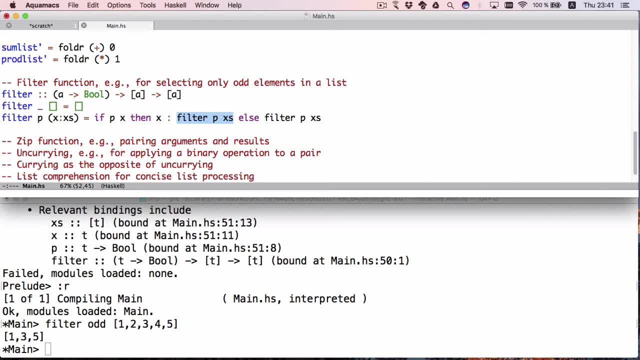 okay, and there's all kinds of clever things we could do. I mean, first of all, of course, we could just factor it. we could have a burr binding where we compute it like this and then we do it like this. this is certainly one option, but actually, 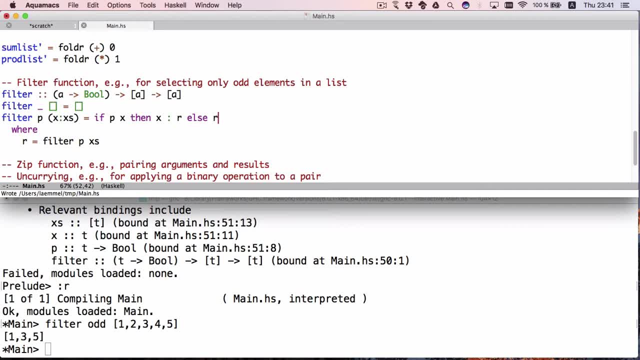 what we might do instead is we might realize that in all the two cases that we face here- the then branch and the else branch- in the end we have to recursively filter the rest. so what we do is we partially apply quants here and here we return. 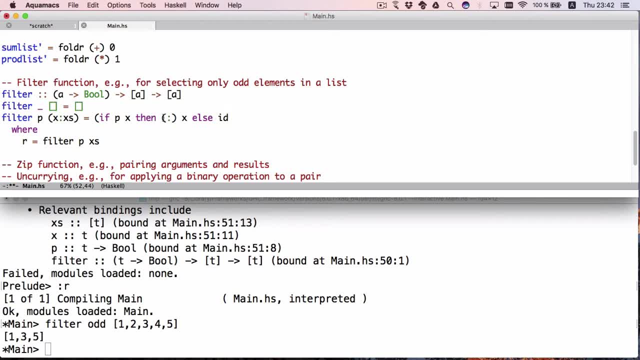 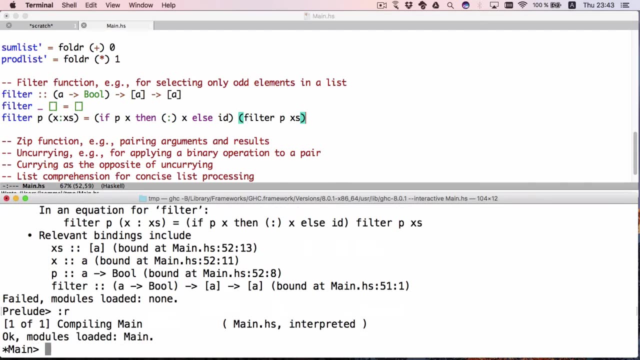 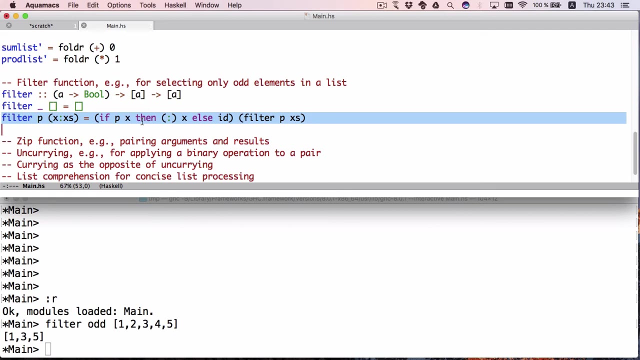 id and we apply this to this filter, alright. so I mean, this is maybe a little bit too clever factoring here, but it's actually sort of nice because it also involves some higher order programming. right, because here we have a partial application of quants, so we still lack the tail. 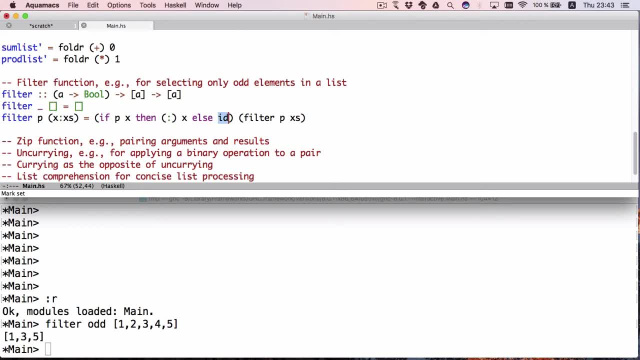 and here for the else branch, there's really nothing else to do than to put in the identity function, which means we will just reuse the recursively filtered tail of the list, as is okay. yeah, there's actually one more function, or family of functions, that we should look at. 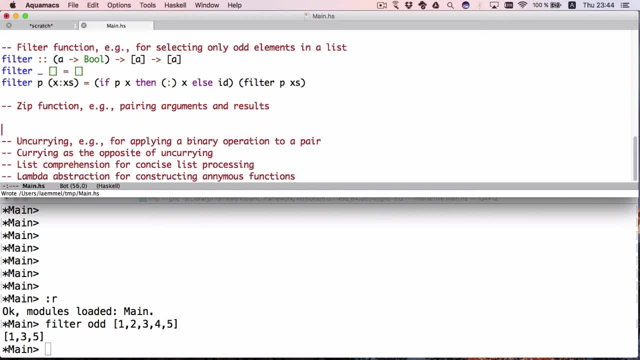 they are concerned with zipping, let's just demonstrate them. so we can zip a list one, two, three- with another list- four, five, six, like this, that is, we form pairs taken from the corresponding positions of the two lists. we can also apply a binary function to those. 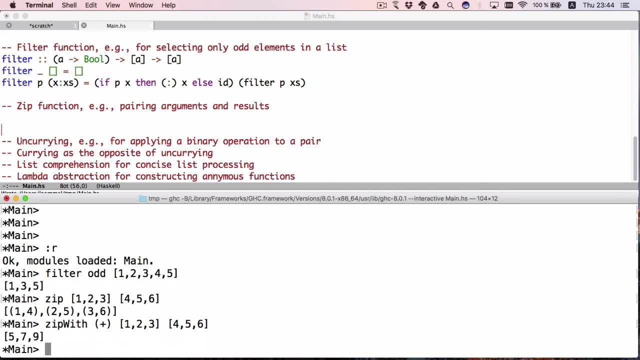 elements. so, for example, we could apply addition. so this means we take the sum of one and four, of two and five of three and six. okay, so these are also very common functions in list processing, because often we need to operate on pairs and, in fact, on list of pairs. so let's just 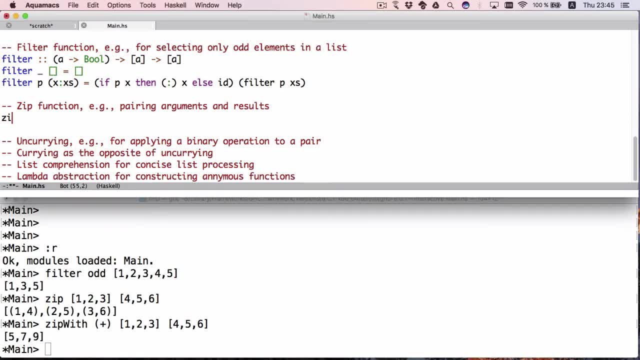 define them okay. let's say z. when we have the empty list here and something here, well then this is just the empty list. if we have something here and the empty list here, then it's just the empty list. if we have x here, x is as well. 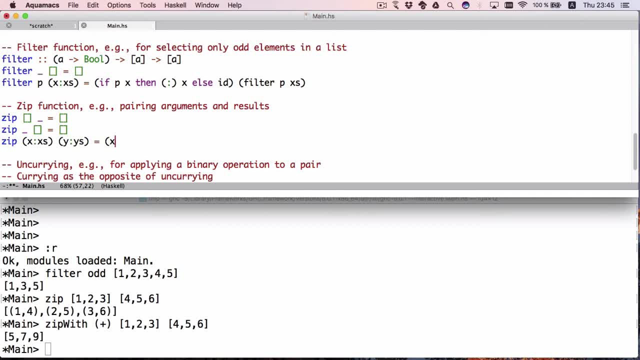 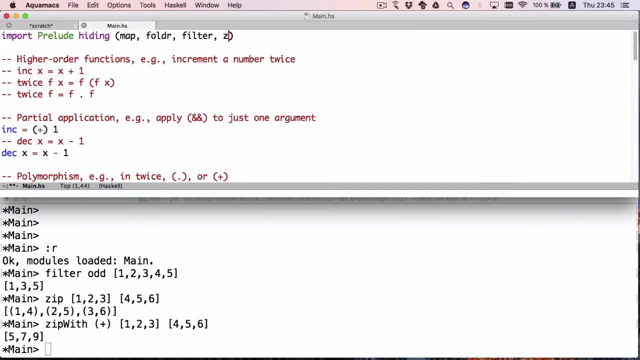 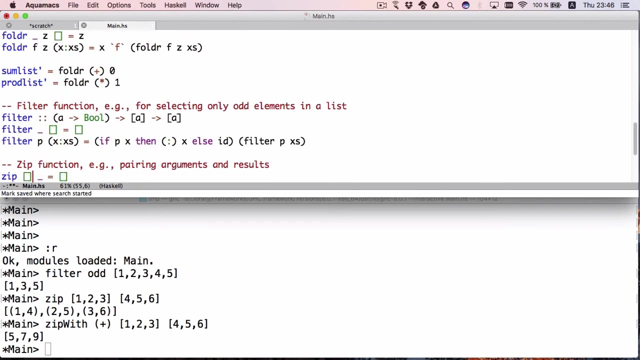 y here, tail y. then what we do is we compute the pair x and we recursively zip together x's and y's. okay, this is the zip function. by the way, we should remove zip and zipwith from the prelude. now, how does the zipwith function work? 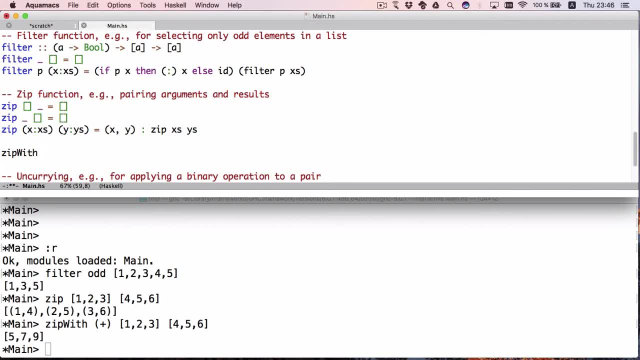 zipwith takes a function, and likewise, when there is nothing left, then we do this, and also here, if there is nothing left, we return the empty list, and if we still have something here and there, then we of course apply f to x and y, and then we recursively. 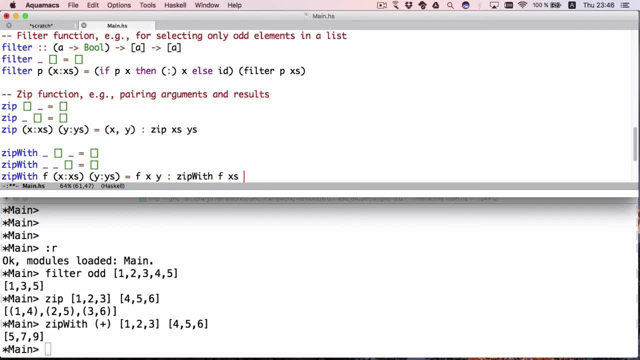 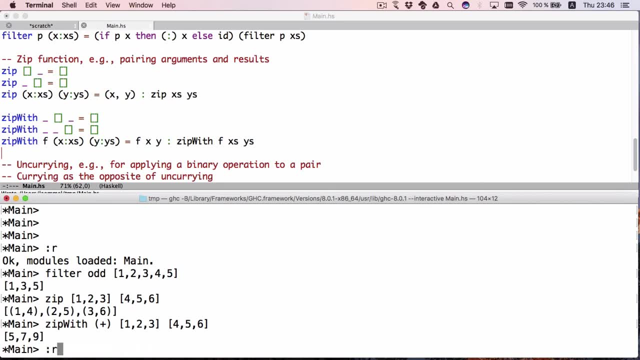 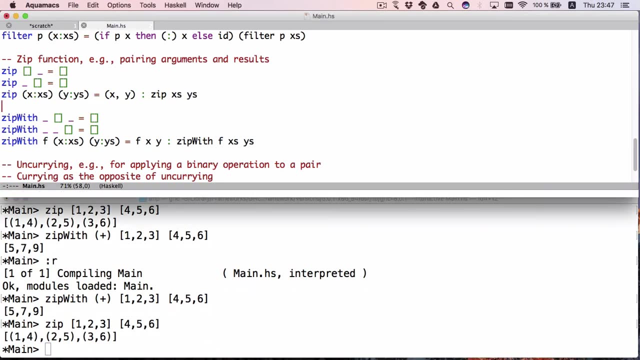 zipwith f on the tails x's and y's okay, still do this and that, and we can also figure out how the types are here. so zip obviously takes one list and another list- they don't need to be of the same element type- and returns a list. 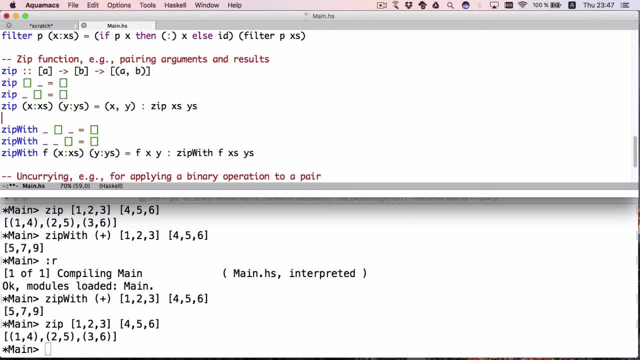 of pairs and here very similar zipwith. we take a function from a and b to c, so and we take a list of a's and a list of b's and we compute a list of c's- okay. so in a way, zipwith is a much more parametric. 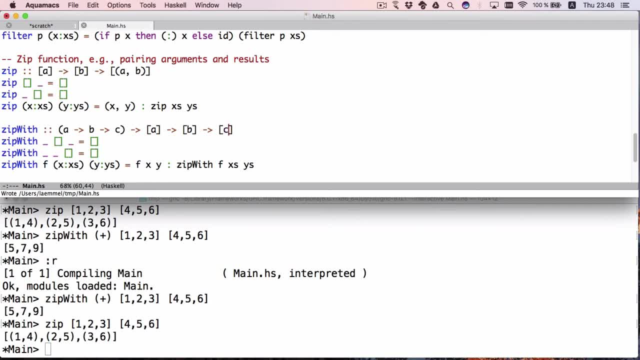 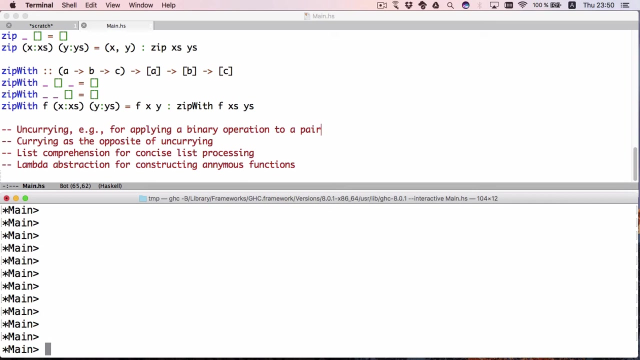 version of zip. strictly speaking, zip is not really a higher order function. zipwith, quite obviously, is a higher order function because we are parametric in what we are doing with the two corresponding elements. okay, let's come to the topic of curing and uncurring. so remember, 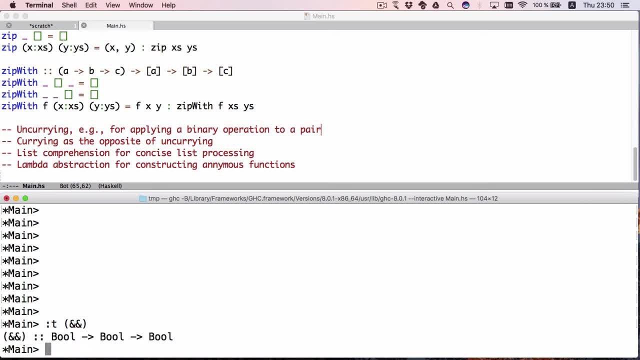 the type of conjunction. it's what we call a curr type, because we first take a bool and then we essentially return something of a function type, and so we take the two arguments one by one rather than in a pair. so there is an operation which is called uncurry. 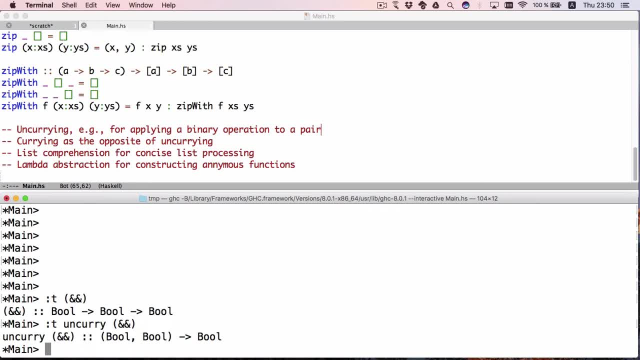 which can massage the type, so that we now see that this uncurry conjunction essentially takes a pair and returns a bool. so this is not completely useless. so imagine we are facing such a list here of pairs- one, two, three, four, five, six- and now let's assume that we want to. 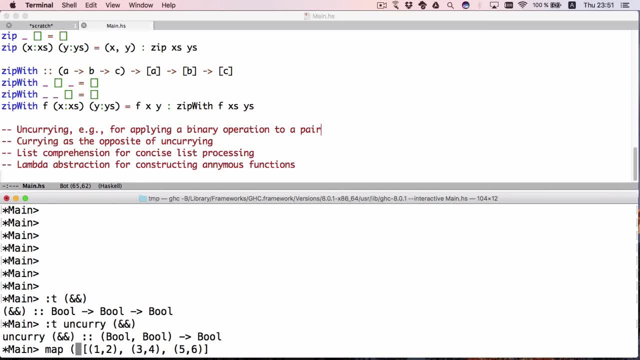 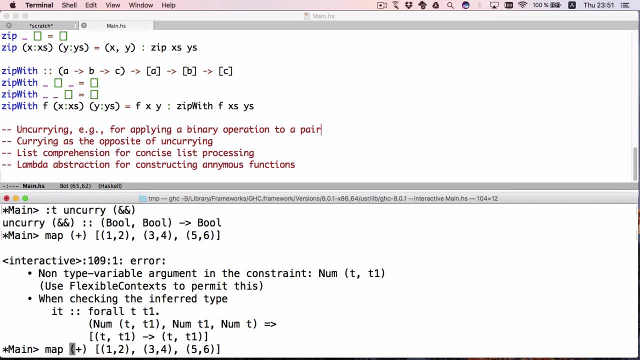 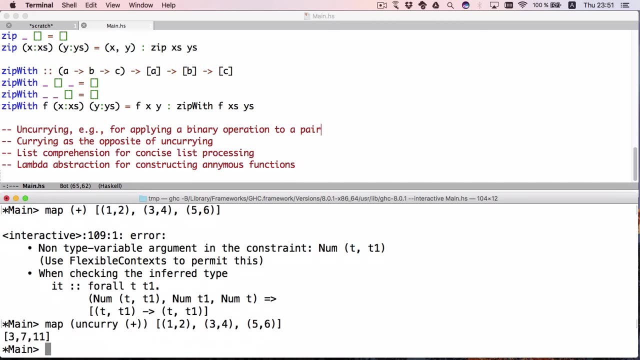 apply addition to this. so if you just write addition here right away, this will not work. however, if we uncurry addition, then this works because obviously, in order to apply to elements of this list, we need an addition that can deal with pairs and so uncurry. 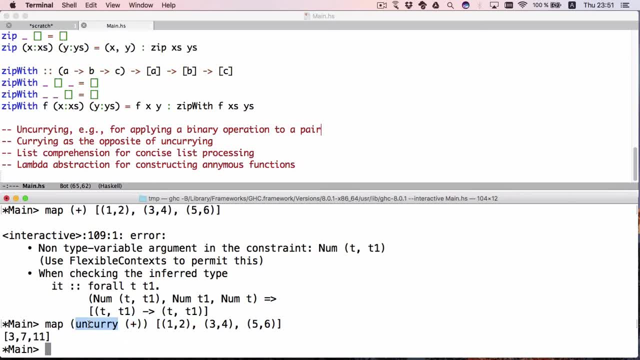 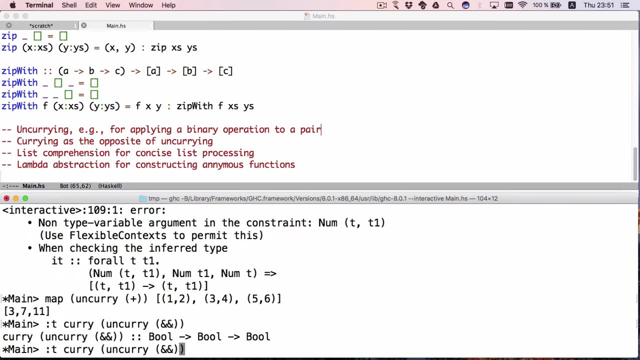 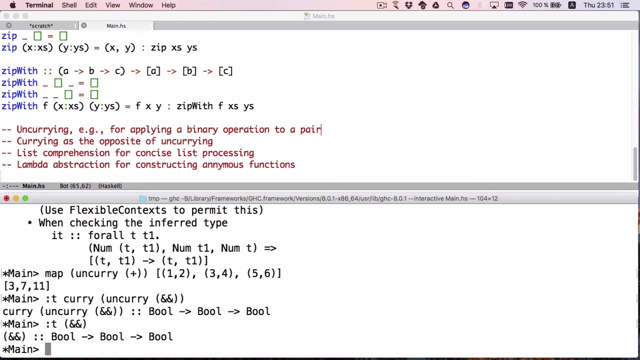 is quite useful sometimes. and there is also another operation which is called curry, which just works the other way around. so we are back to the original type of conjunction. so this is the same type as this and it is pretty easy to understand how currying and uncurrying works. 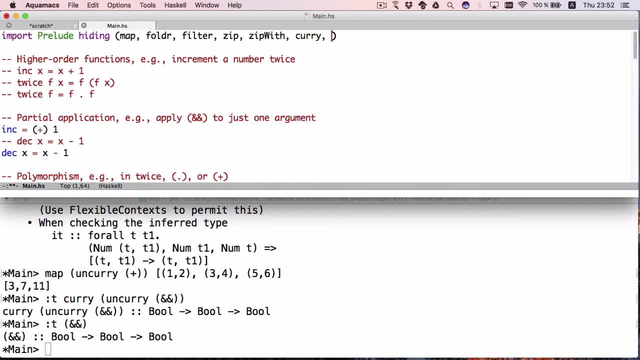 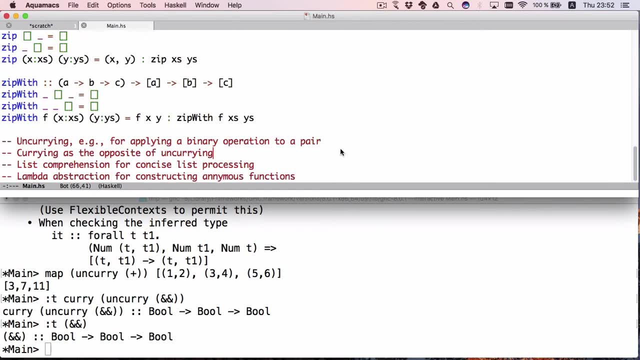 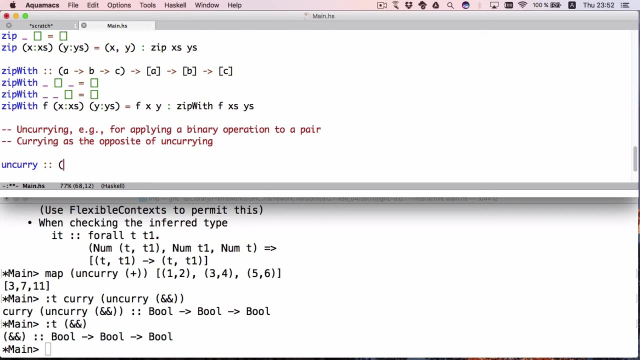 so again, let's hide it and let's go here. so uncurry, as we said, takes a function from a to b to c, a function with two arguments, and turns it into a function that takes an a and a- b as a pair and returns a c. 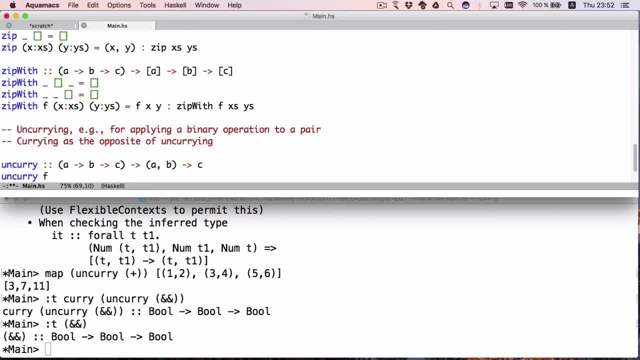 and what we do here is we just receive the argument, the pair, and then we just apply f to x. likewise, curry is supposed to work the other way around. it takes a pair a, b and in fact a function on such a pair which returns c and it. 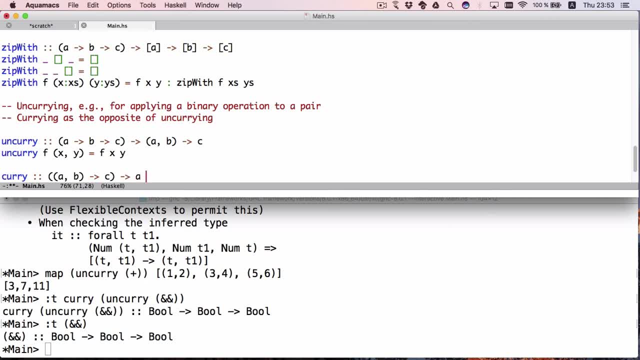 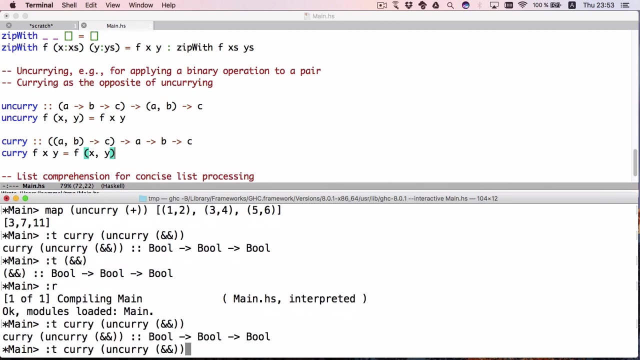 returns something, a function that takes an a and a b and returns a c and curry. what we do here is we just receive an f, and so we need to bind x and y, and we just apply f to x and y. okay, so this is still the same. 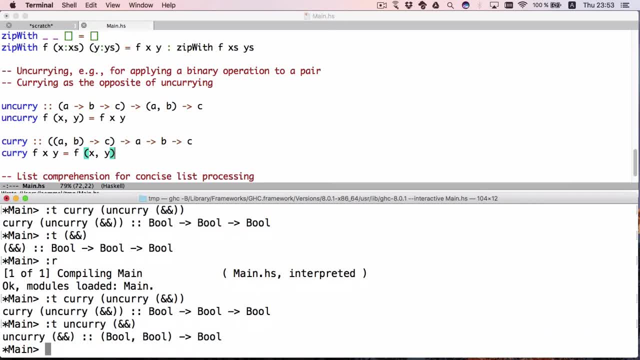 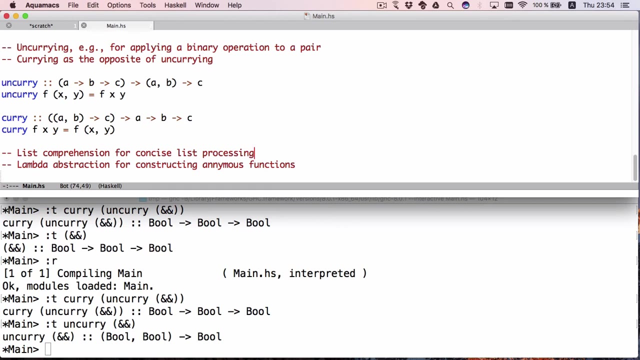 as before. right. this also explains how we can go from functions that take arguments one by one to functions that take their arguments as pairs or, more generally, as tuples. now a few more things. rather than just working with map and filter and such list processing functions, there is also an alternative. 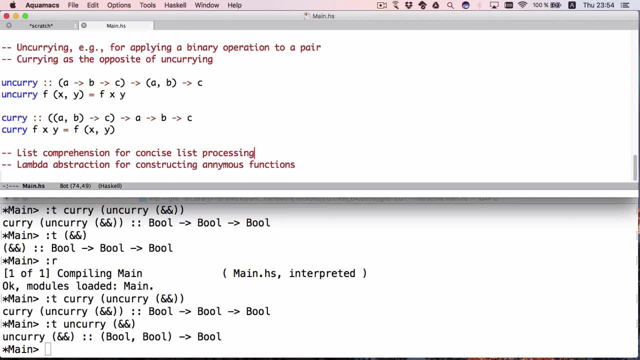 notation in Haskell- and also in other functional programming languages for that matter- which is very concise and which is inspired by mathematical set comprehension notation, which allows you to describe concisely how you form new sets from existing sets. and well, in Haskell it's about lists rather than sets. 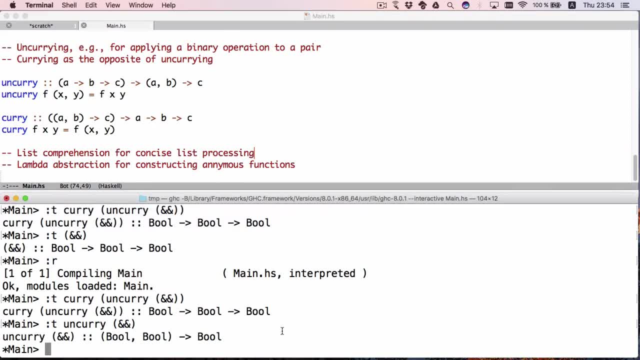 okay, let me just show you how this works. um, so we basically use kind of list notation to perform list comprehensions. let's just say we do something like this. this is a very stupid example. what we do here is we say for the list of all the x's. 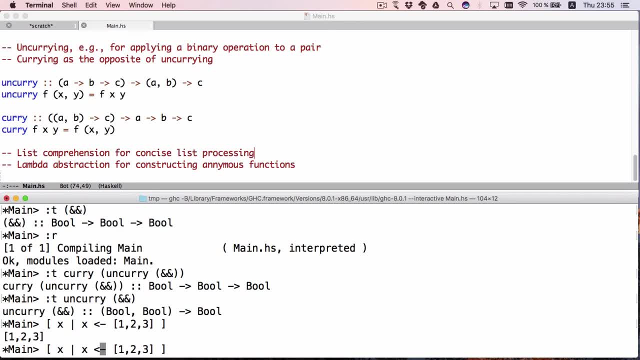 where x is drawn from 1 to 3, okay. but we can do something else. we can say for the list of x plus 1 where x is drawn from 1 to 3. so you see, this is actually a little bit like a map now. 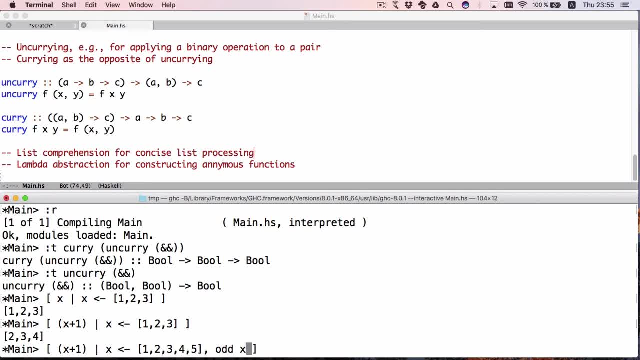 let's add a predicate here. so now what we do is we form a list of x's plus 1, such that the x's are drawn from this list. 1, 2,, 3,, 4, 5, and the x's also need to be odd. 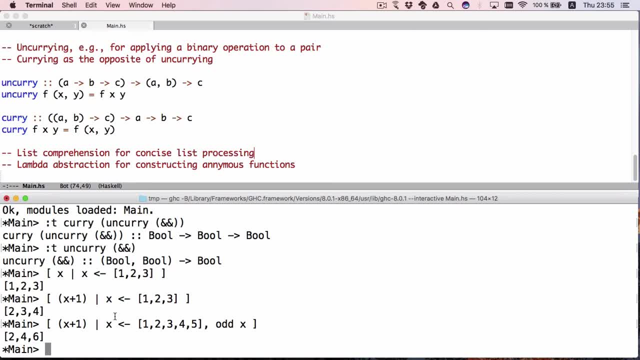 okay. so this means we can very concisely combine sort of mapping and filtering, right. so in terminology of Haskell we call this sort of expression here a generator, because it generates possible values for x, and this we call a guard, because it kind of defines a guard. 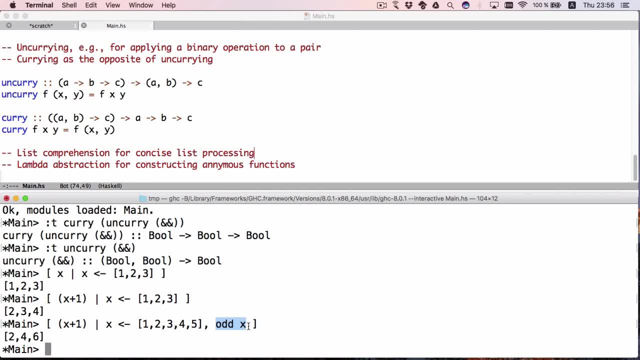 on what values well survive. let's say: we can do many more things here. so, for example, we can also have multiple generators. so let's say, x is taken from 1 to 3, whereas y is taken from a, b, c. what we get here is obviously: 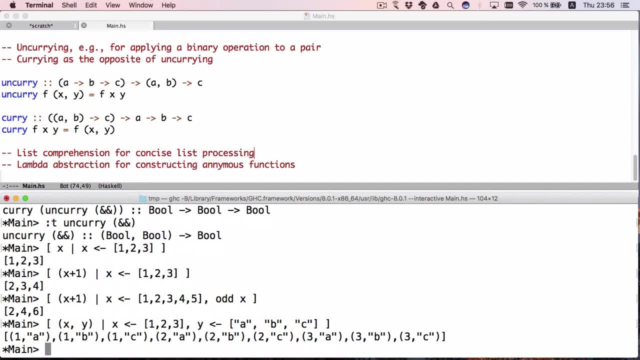 a list of all pairs, of all possible combinations of elements from x and y. so this means we can also do this sort of combinatorial list processing, which would not be so straightforward when just using map and filter and such. but actually as an exercise you might just. 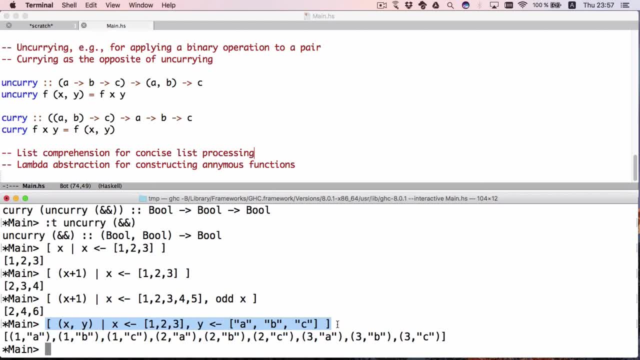 think of how you express this without list comprehensions. okay, so basically, Haskell programmers like to use list comprehensions when they want to, when they have more complex patterns of how different guards and different generators interact, rather than using list processing combinators directly. okay, there is one more topic. 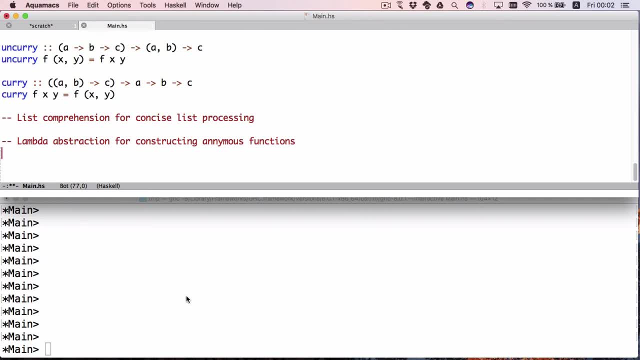 that we should cover here the notion of lambda abstraction or anonymous function. so let's just revisit some of the examples we have seen earlier. so here we defined a stupidly simple function increment. or here we defined a stupidly simple function decrement, and then we were using them.